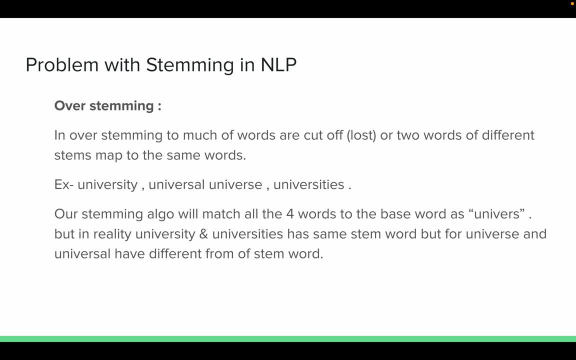 The first problem is the over stemming. So what are over stemming? The over stemming in which the two words with the different meaning just map to the same stem. So I can just give you the example so it will be like more clear to you. So you can just take an example of university. So university and universal, You know that this both are meaning is different. University, if you are going to for stem word or the root word of university, it will be university, That's it. And for the 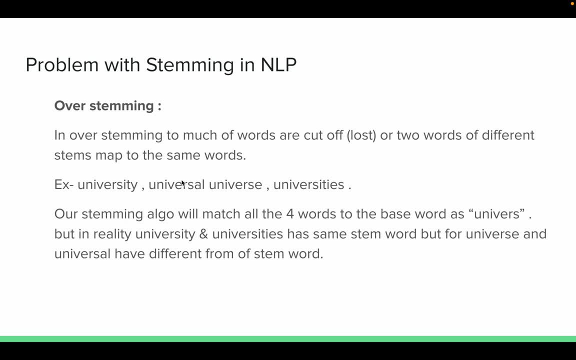 universal will be universal, That's it. But here, if, whenever you are going to use the stemming in this particular natural language processing, you are going to match the root word of the both university and universal as the same, So it will just match as a universe. This will be the output. So for the all you can just say university, universal universe and universities. They will match to the same stem word, that is a universe. But you know that university and universities. 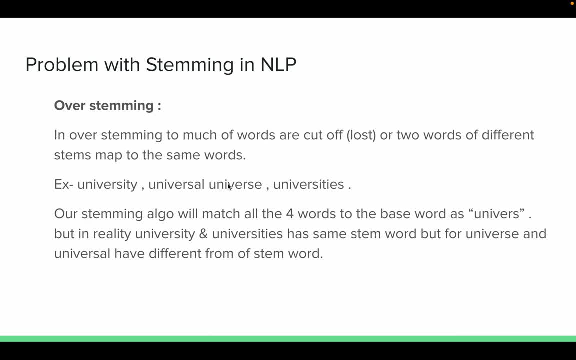 This, both stemming word will be the same And for the universal and universe the stemming word will be the same But for all you are just getting the same root word or same you can just say base word. So there is a problem with the stemming. This is called the over stemming means. whenever you have two words, You have two words. that will. you know that that belongs to the different stem words. But whenever you are using the stemming techniques the root word of both will be the same. So that is really problem in the stemming. 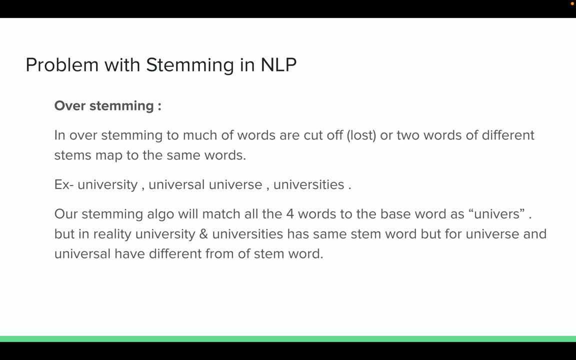 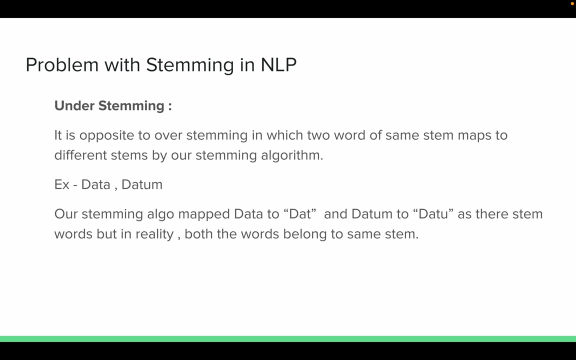 You can't directly go for the stemming and then after you are going for you are just creating any model. So it may give you some error because you are just converting stemming that particular university and universal with the same stemming that a universe. So this model will treat as universal and university as a same. So this is the problem of over stemming. Again, we will see this thing in the practical part also. And the second thing is the under stemming. So under stemming is basically opposite of the over stemming. 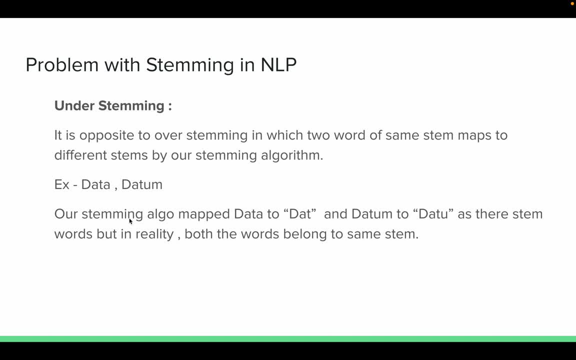 Okay, In this under stemming, whenever the two words. you know that the two words with the same should be same stemming stem name. Okay So, but here it will give you the different, different stemming name. Okay, So, what does stemming name? I'm just saying I will just give you with the again, with the example, So it will be more clear. So you can just, first of all, you can just see the theory also, It is opposite to the over stemming. that already I say you. Okay, That is the two word of the same stem maps to the different stem means. whenever you have, you are trading, you are just creating two words. Okay. 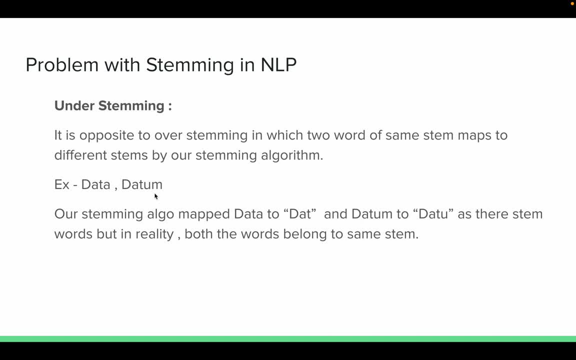 I'm wrong. Okay, Are you Data and science? Okay, This two words unit of books stem worked out which one of the beast, both will be the same. That is the data, Okay So, but here, If you are just writing this, you are just using the sterling algorithm and you're just applying for the data and later on you're going to know the base. What are doing, bolded off that they gave you a different based on that different thing. but for the beast, both Okay. 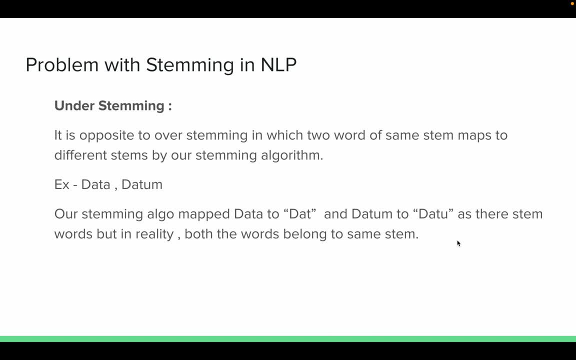 And for data. we will give that. Okay So, but you really know that? the stream, what about that Meaning Of both really the same, okay, so originally we are calling as a datum and now we are just calling as a data, but the steam word of both should be the same, but here in the under sampling: 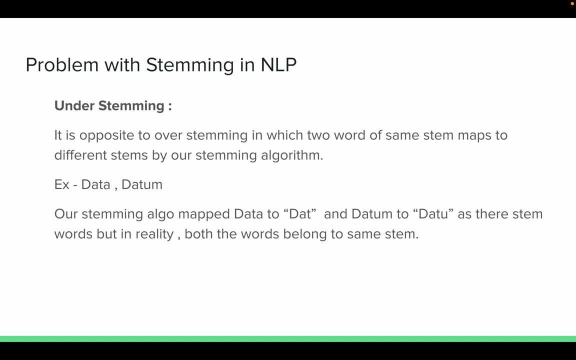 the two words will give you the different steam name. okay, this was the problem. and in the stemming: okay, so i hope. so you are clear with the over stemming and under stemming. okay, so we will again, we can just look in the practical part also if you want to go through. so first of all, what you 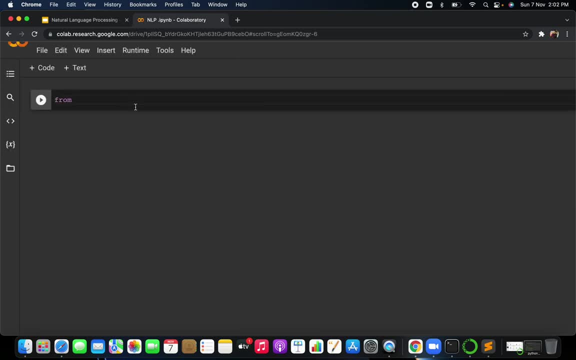 can just import the library we are going to use. we can just use porter streamer. that's it from nltk dot stim import porter. okay, so porter streamer, and then after make the object of that, leave it just run first of all, if it is not giving an error now, just create the object of that, okay. 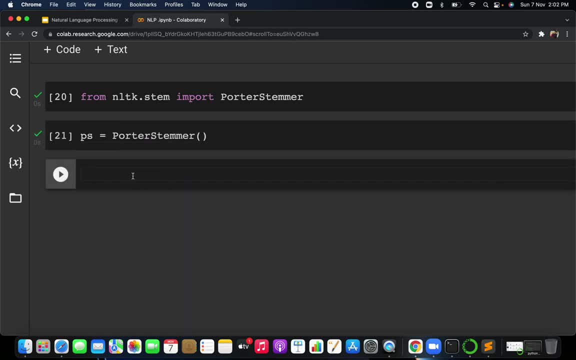 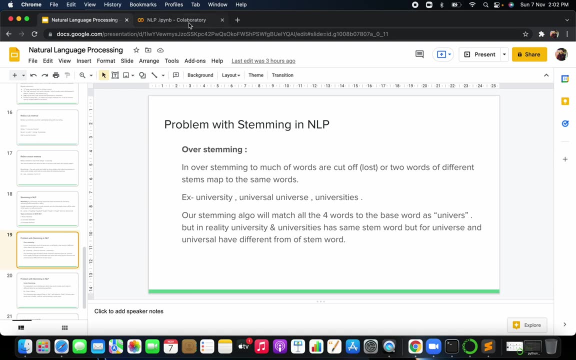 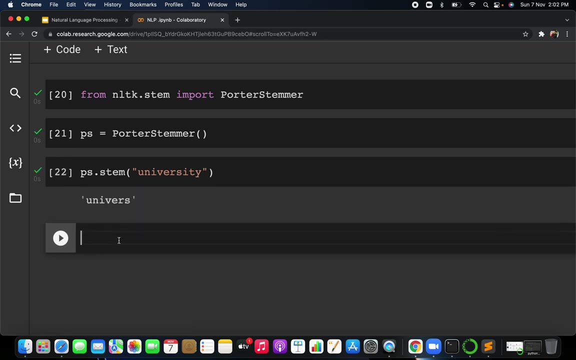 then after you can just see if you want to do the stemming of, you want to do the stemming of university, okay, the first we already seen. if you want to do for university, okay, university, then what will be the answer? university, okay, and just see: ps will give you universe, okay, that's what. already i will explain you: universe, so it is. 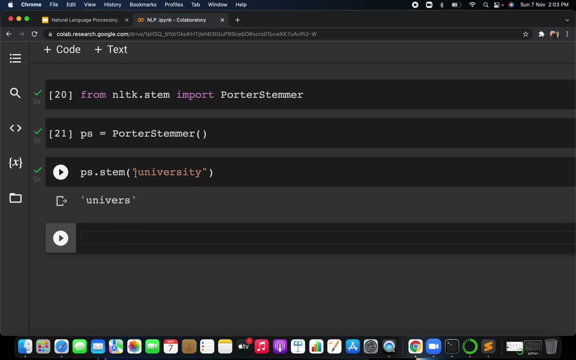 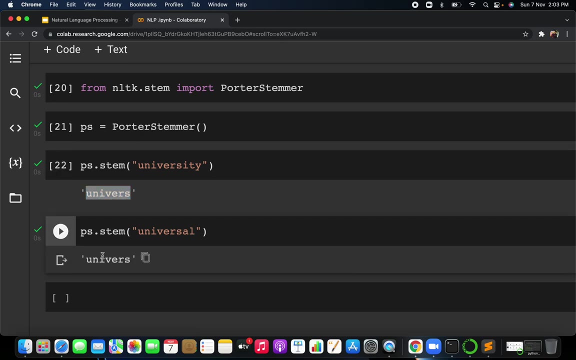 really, really wrong. you know that university is a different thing, but universe is different. okay again. you want to try for the universal? okay, universal, you want to try for universal. so what will be? it's again the same universe and universe. okay, so this is the problem in the 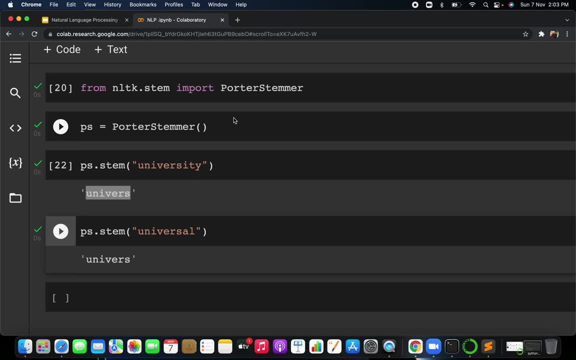 particular over sam, over stemming. okay, so what? over stamping? i think you are clear. okay, the two words with the difference in the different stemming where they match to the same base word or the stem word. okay, so this is the really two different word. okay, this university is different word and. 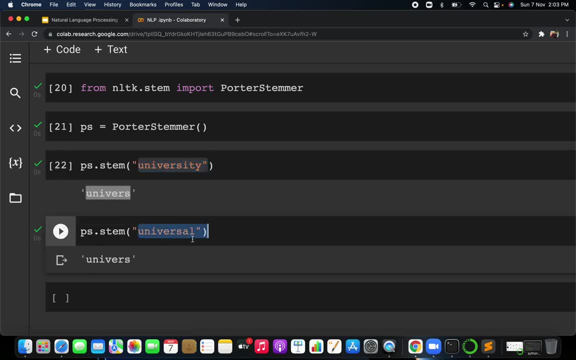 universal is the different word. okay, but you, this particular, whenever you are applying the stemming algorithm, the their base word or root word is match as the same. okay. so this is really blunder. you can just say: because whenever you will fit to, whenever you are creating any model and you are, 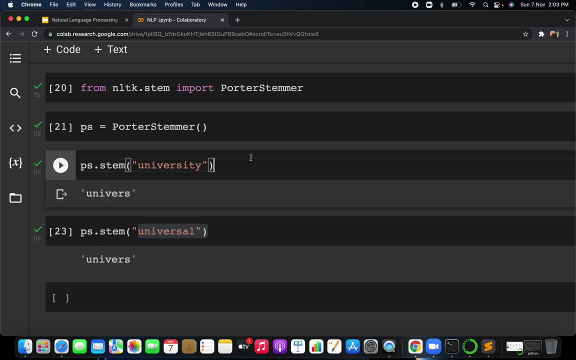 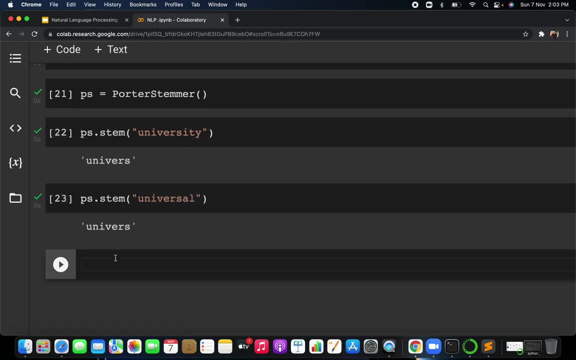 just treating university and universal as the same. so it may give you an. it will not give you an exact accuracy. okay, so this was the problem of over sampling. okay, so this is the problem of over sampling, over stemming. so this was the problem of over sam, over stemming. again, you can just try for the. 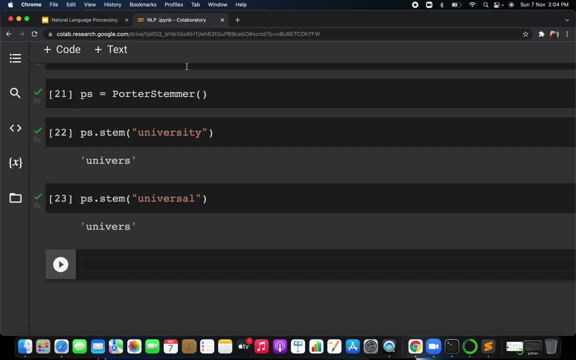 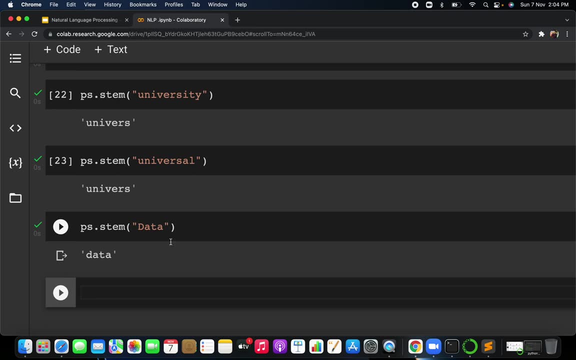 particular we have seen for the under stemming also. okay, so you can just try for the same stem. and you want to try for the data? okay, so, data, i can just write. so what will be the output? it is basically the data it is giving you and then after, if you will try for the datum, okay, datum. 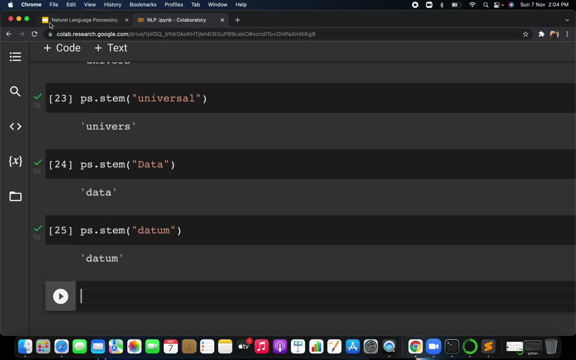 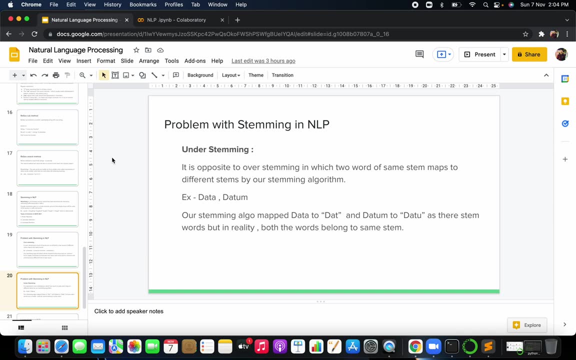 datum. okay so, basically, it is not giving the exact accuracy what we are going to use. okay so, basically, so, basically, the what? what is the problem with the under sampling that two? basically, what will match to the two different words? because you know the data data is really the same. okay so, but there, 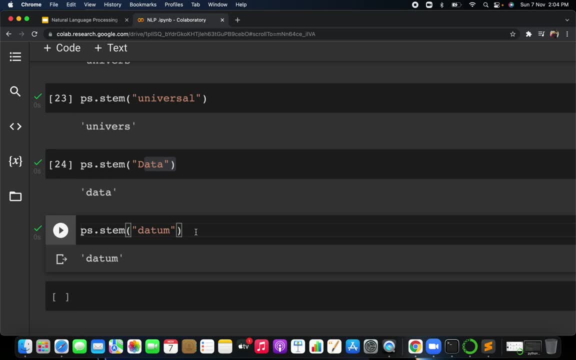 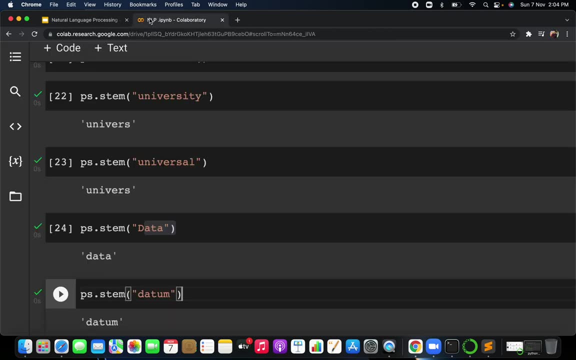 should be same stemming word, okay, the root word. but here it is giving you different for the different of words. okay, so this is the, basically the under sampling. so i think you are clear with the same in the basic. i can just say you over sampling in which two words, two diff, two different word. 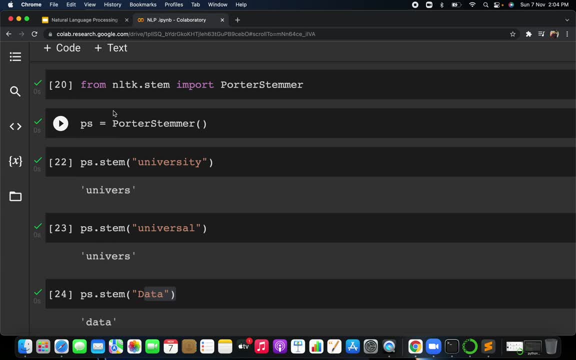 so is matching with the same stem word, okay. base word: okay. that is the problem. and under sampling means two same word is matching with the different stem words, okay. so this is the uh problem. we already seen in the under sampling and over sampling. so in the next video, how to come with this solution or this problem- we are going to.